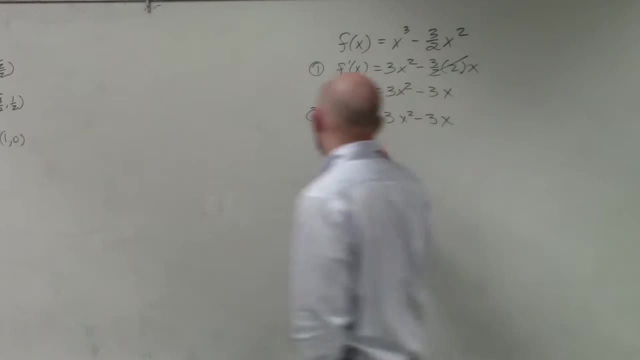 We see this is a quadratic, so we're going to want to use our factoring technique. Zero equals 3x times x minus 1.. So we could say: by applying the zero product property, you could say x equals zero and x equals 1.. 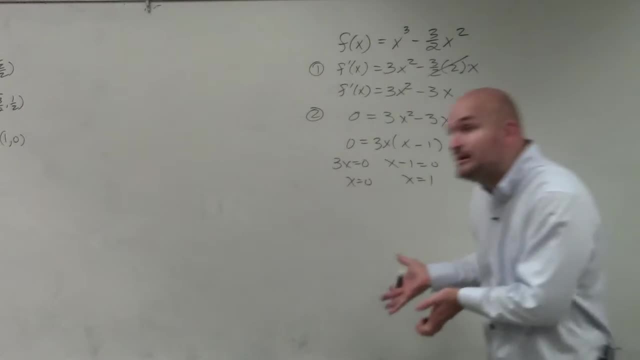 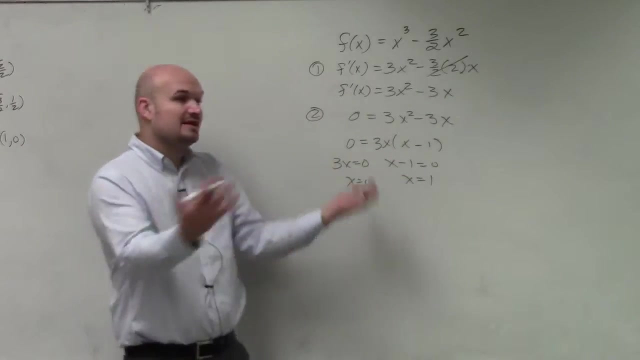 So those are our critical values, right? Those are our possible extrema. All right, We got to be able to make. that's where the horizontal tangent is. We have a horizontal tangent at these values. They could be our max and mins, but we have to be able to test. 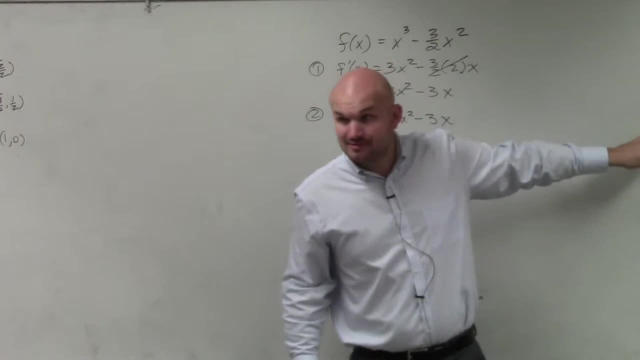 We don't just want to assume- because remember, there was that option three, right, There was that option three- that it can change from positive to positive. So just because you have here, don't assume that these are going to be a max or a min. 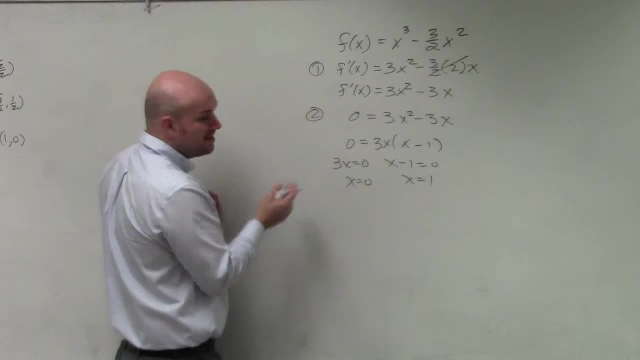 We have to go and test our intervals. Now I'm going to show you one thing to me that makes sense, but I don't want you guys to use it on your exam. I'll show you guys what I'll have you guys do on your exam. 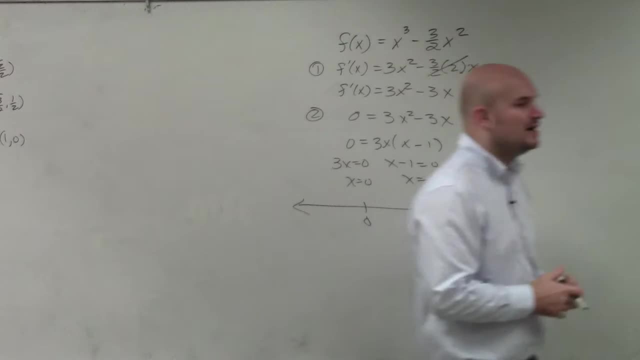 But I just want you to know I'm going to show you one thing to me that makes sense. but I don't want you guys to use it on your exam. I just want I like using this and I taught this for vertical motion because it kind of just makes sense to me. 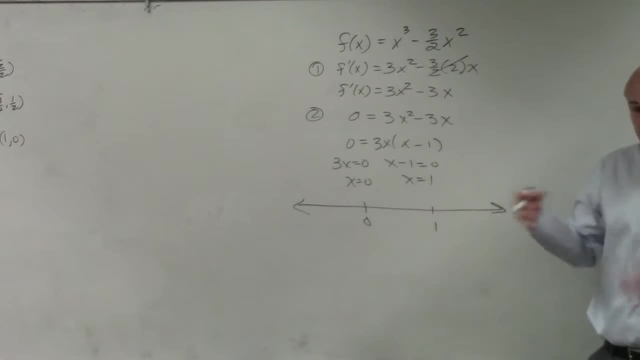 You have your number line right. You know, here is your extrema. What we need to do is identify if f prime of x is going to be positive or negative. We know, at this value and this value, x is going to equal. 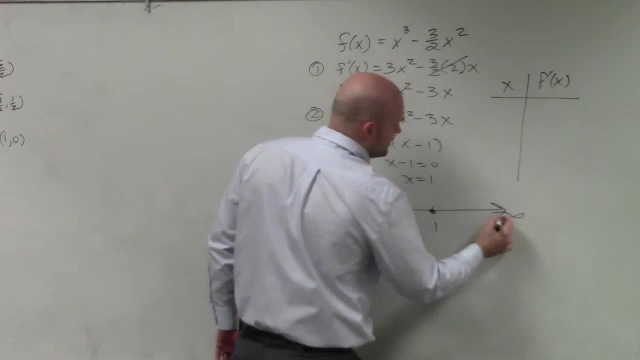 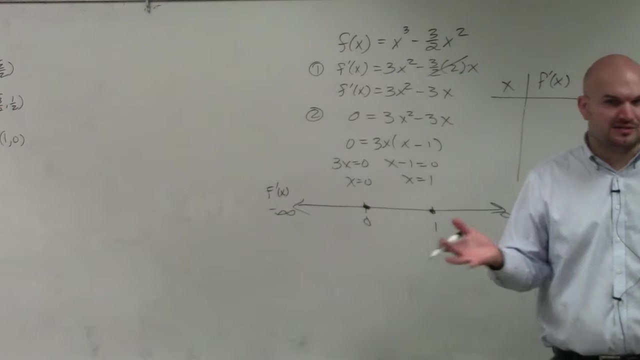 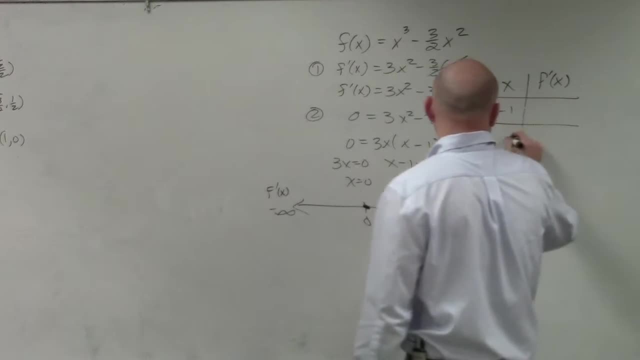 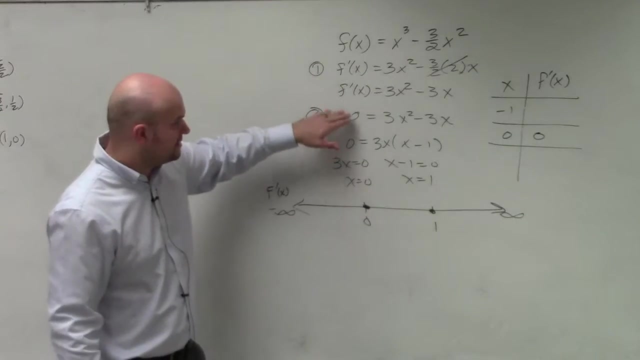 And probably a good number. to be simple, I would say it would be negative one At zero. we know that at zero, f prime has to be equal to zero, right? Because that's how we found those values. I need to pick a value in between zero and one, so I'll pick one half. 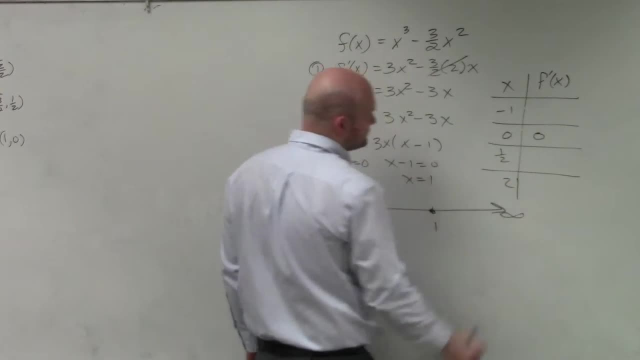 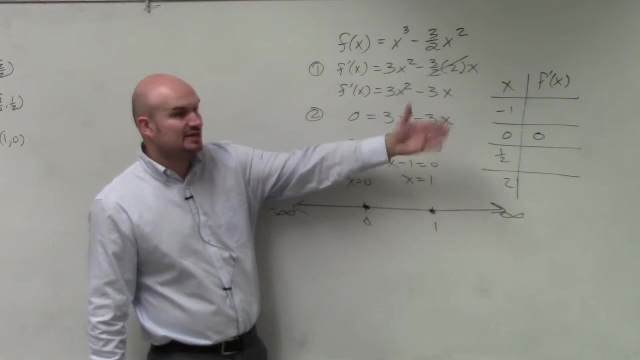 And then I need to pick a value after there, so I'll pick two. Okay, Now, basically, what we need to do is we need to pick a value in between zero and one. to do is plug in negative 1 into our derivative function. 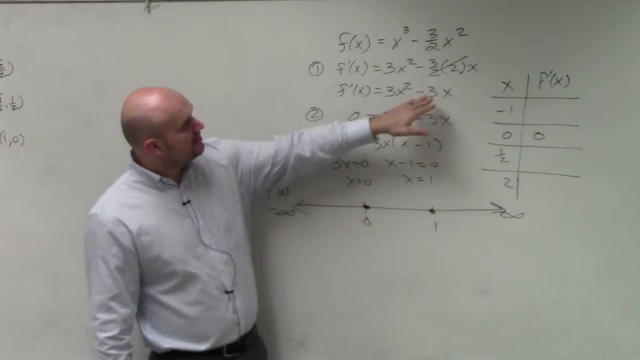 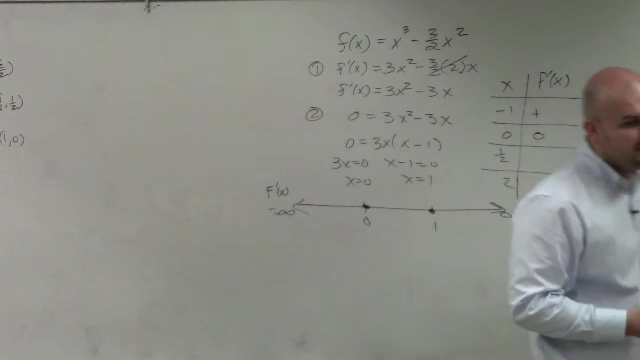 and determine if it's going to be positive or negative. So if you plug in negative 1, that becomes positive, That becomes positive, So we could write positive. It's a simple form, But a preferred mathematical notation would be: f prime of x is greater than 0.. 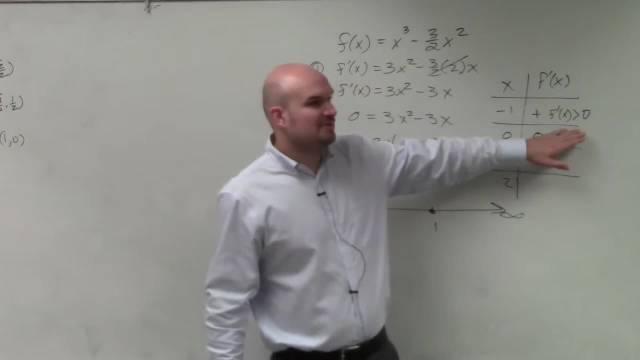 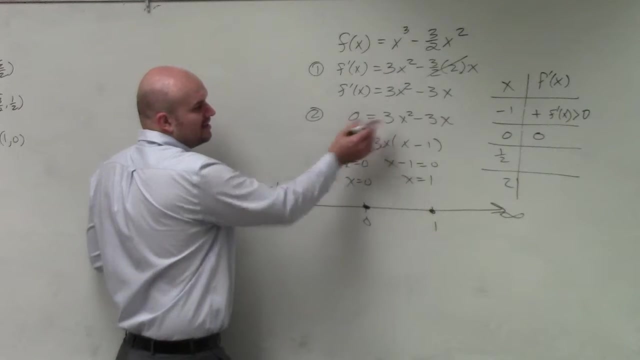 So I'll use positive for it to kind of make sense. But we would prefer to be using mathematical notation, especially with taking an AP exam At 1 half. let's just go ahead and plug that. So 1 half, that's going to be 1. fourth: 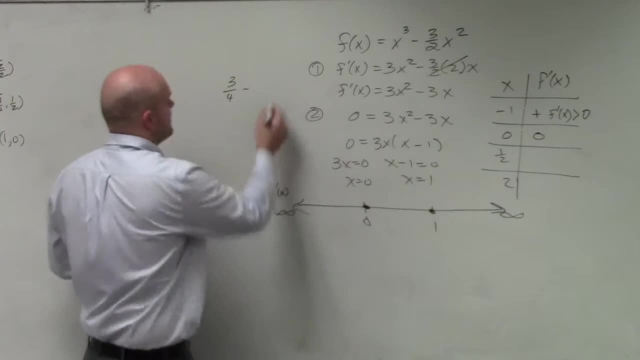 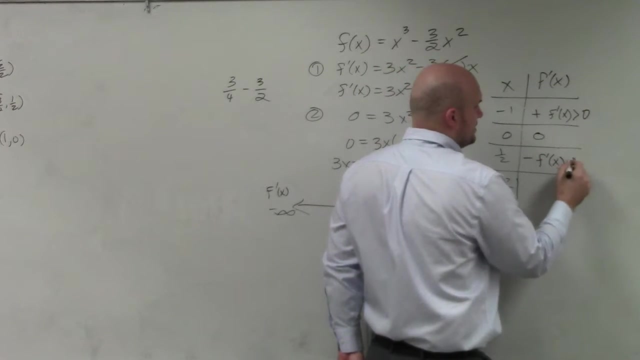 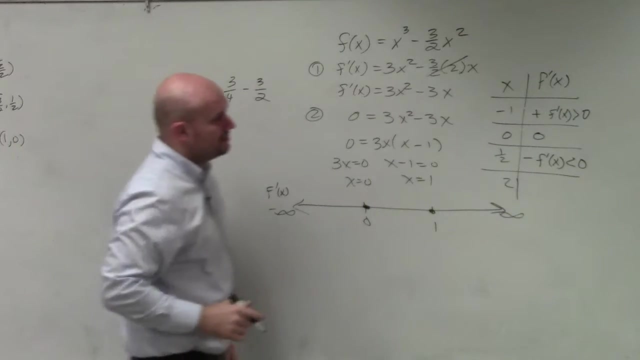 So you'd have 3 fourths minus 3 halves. So that's going to be negative, or f prime of x is less than 0, because 3 halves is larger than 3 fourths. And then we go ahead and plug in 2.. 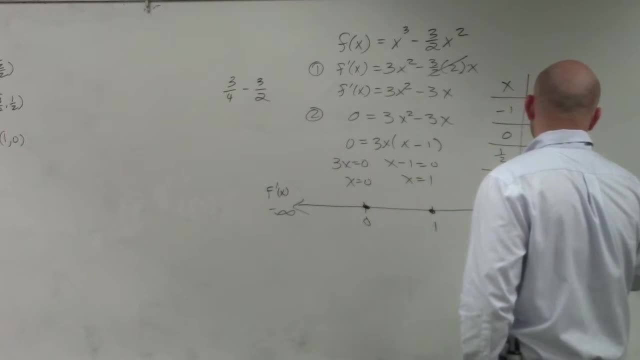 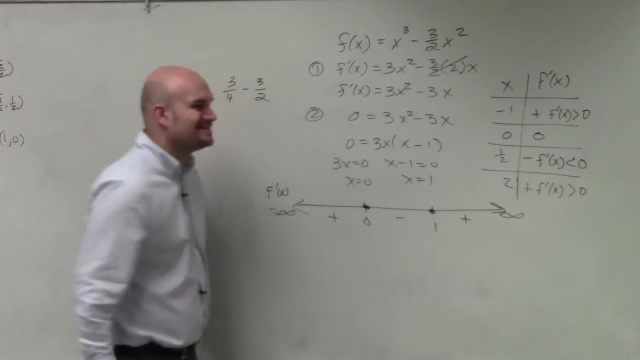 And you guys can see that that's positive. or f prime of x: It's greater than 0. So the way that it makes sense, we're looking like this, But you do not want to use this as your justification. Basically, I'll do another problem. 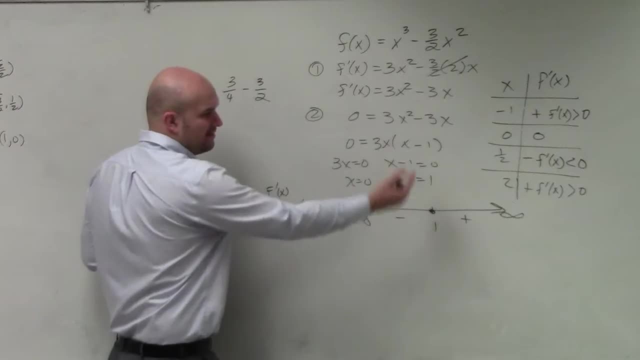 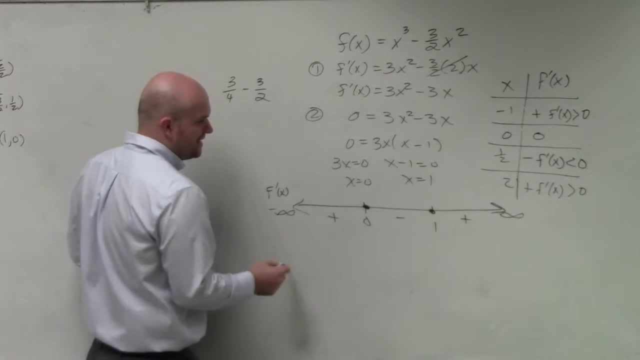 where I'll show you the justification of how I would write it out. But I want to kind of show you guys this way so you guys can kind of relatively see what the process would be. So we can say: you guys can see that it's increasing. 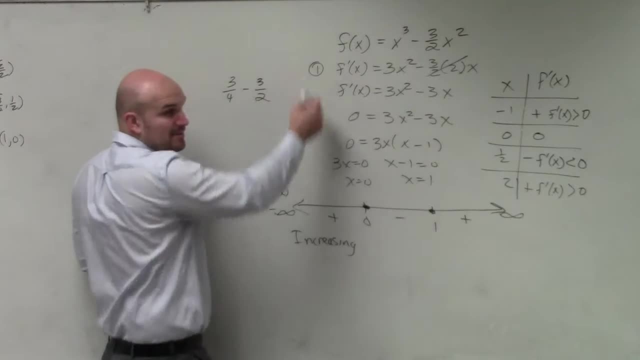 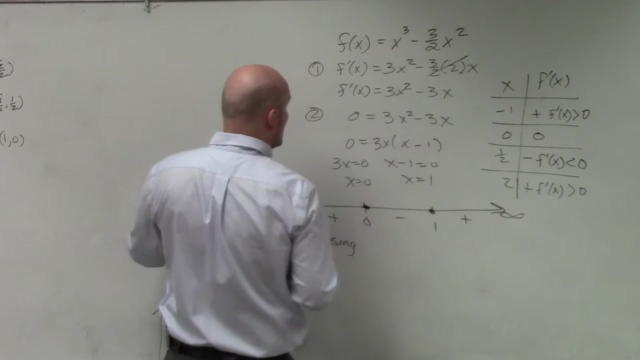 on two different intervals, Right, Remember, I just wrote up there. Wherever the derivative is positive, we know the function is increasing, Just like how we kind of talked about velocity. So it's increasing on the intervals negative infinity to 0, and on the interval 1 to infinity. 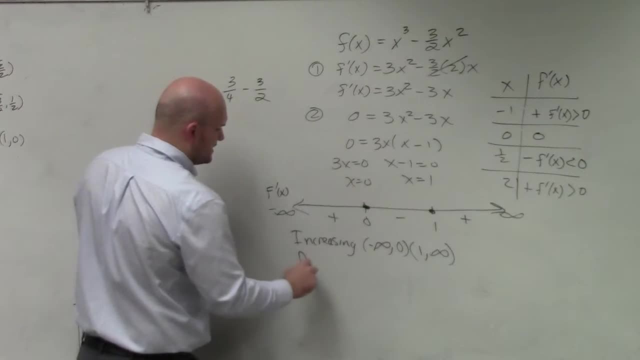 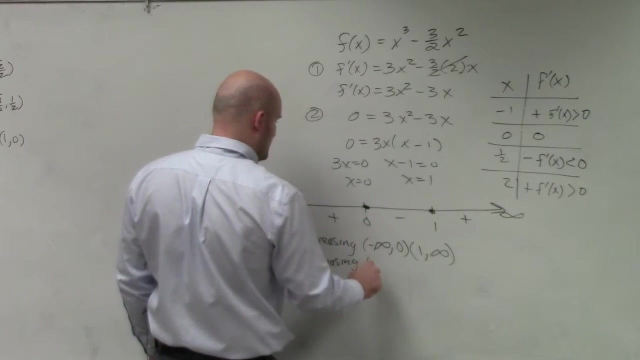 You could also use the union to connect those if you wanted to. It's decreasing on the interval of 0 to 1.. And I am going to write this in nonunion, in perfect format for you. You could also say that you can see from here to here. 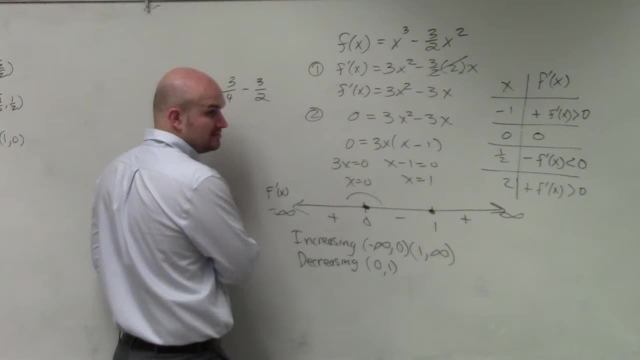 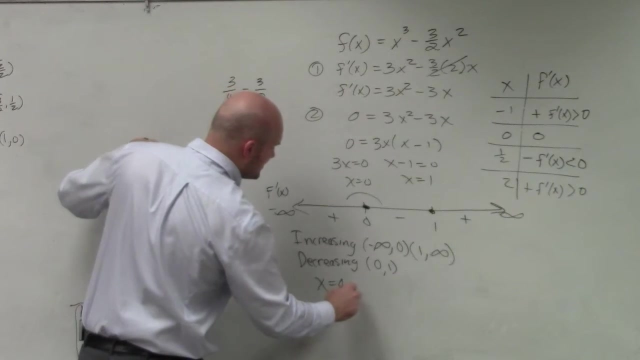 it changes from positive to negative, So it changes that positive, negative. So we could say: at x equals 0 is going to be a. let's see positive to negative, That's going to be a relative max. And at x equals 1 is a relative min.